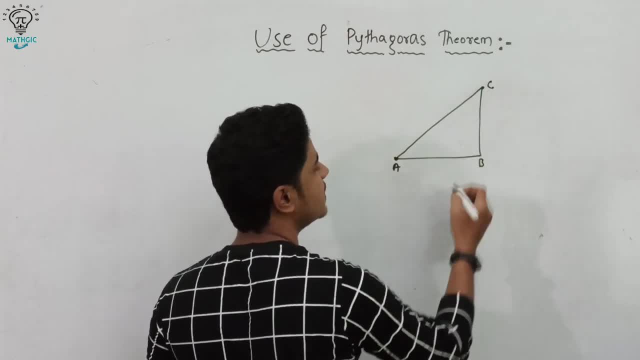 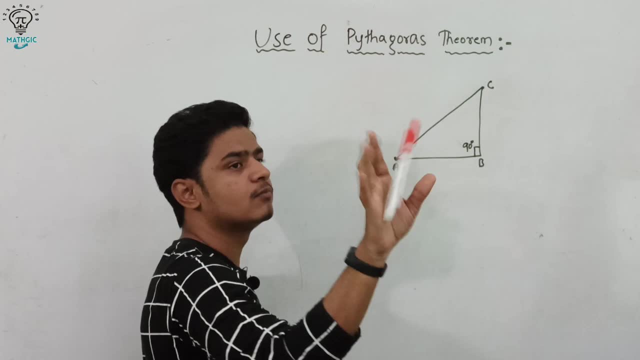 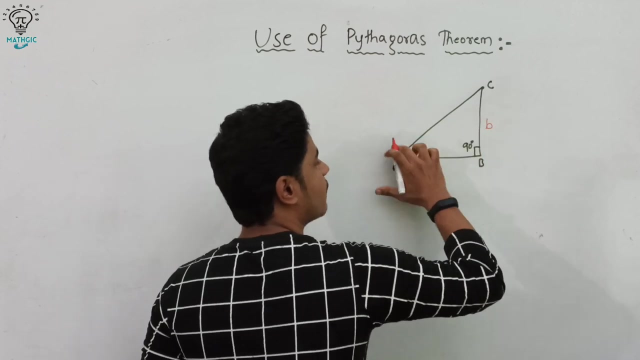 point A, point B and point C and the point B must be 90. degree means right angle triangle. So the length from A to B let A, and from B to C B and from A to C, C, A, B and C are. 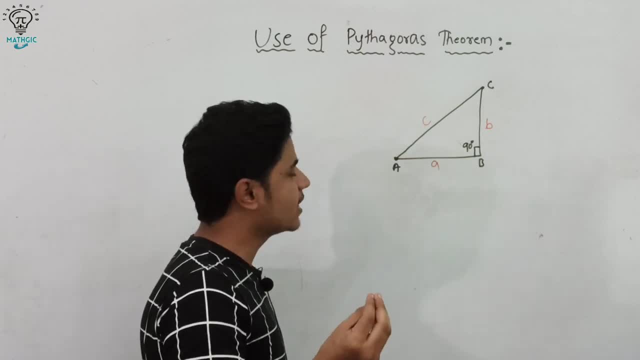 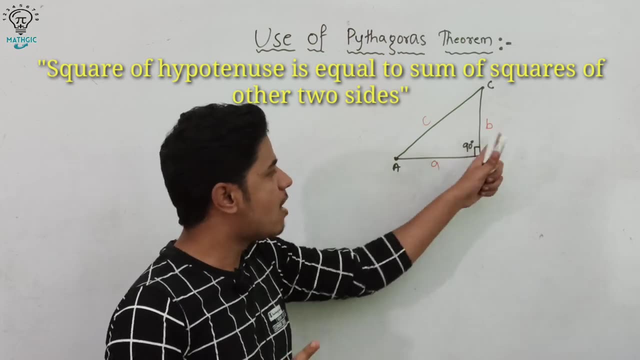 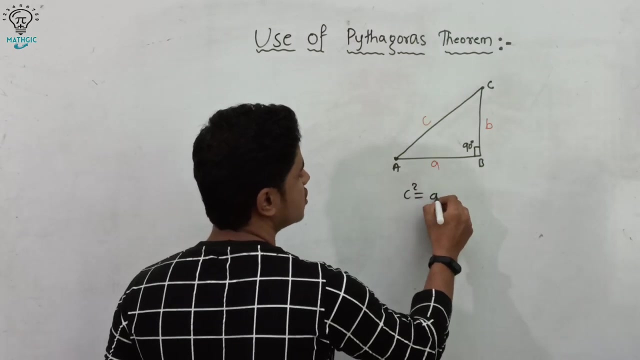 magnitudes must be in kilometer or in meter. So Pythagoras theorem says: square on the hypotenuse is equal to sum of squares of two other sides. So it means C square is equal to A square plus B square. So this is statement of Pythagoras theorem. So let's have an example. 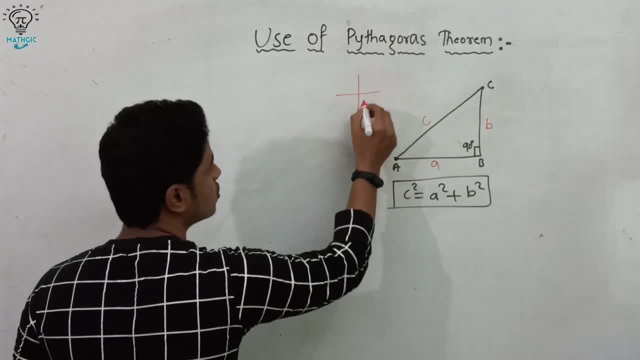 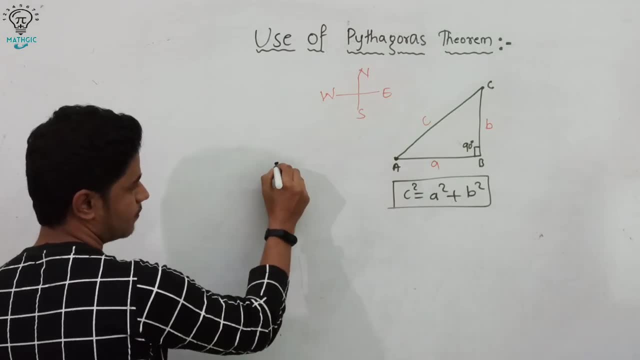 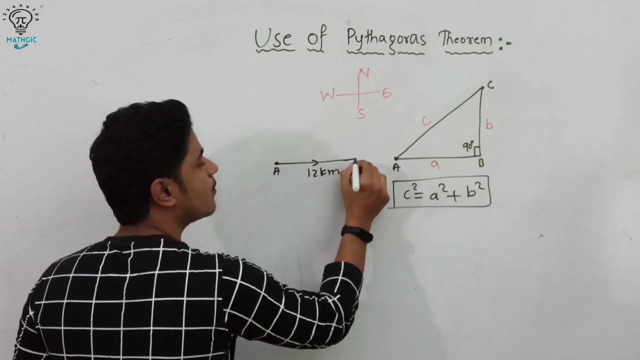 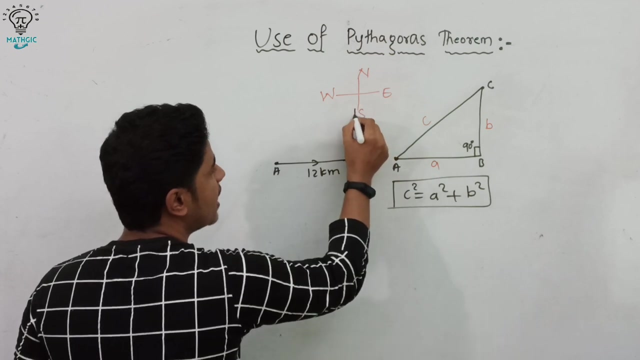 of that. So draw the direction first South, north, east and west. A person went from point A, from point A towards east, 12 kilometer To reach point B. To reach point B and from point B towards south, 9 kilometers. 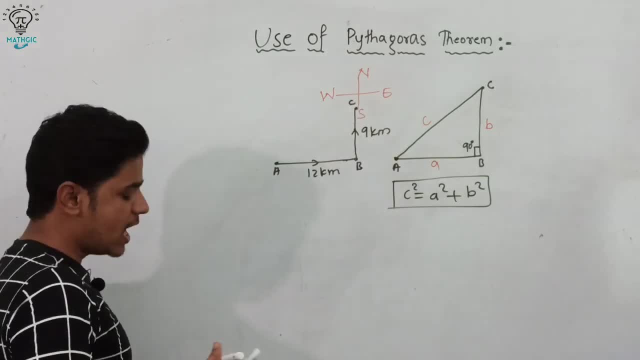 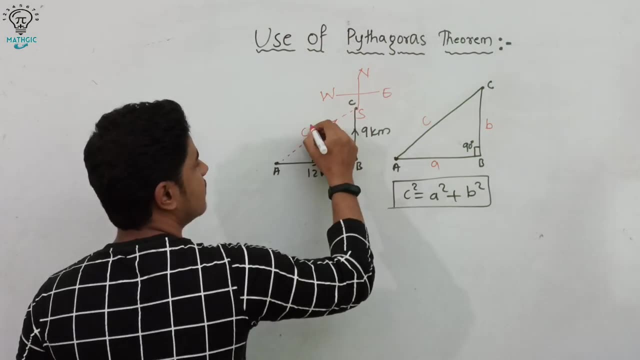 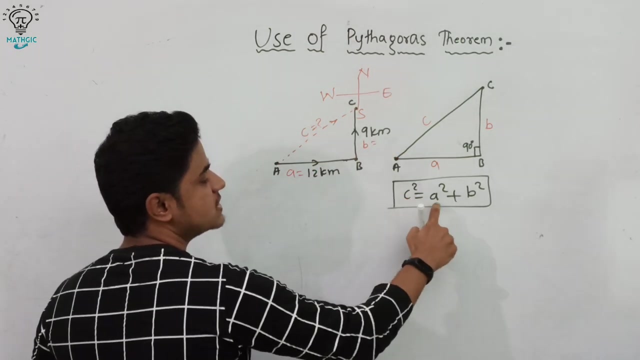 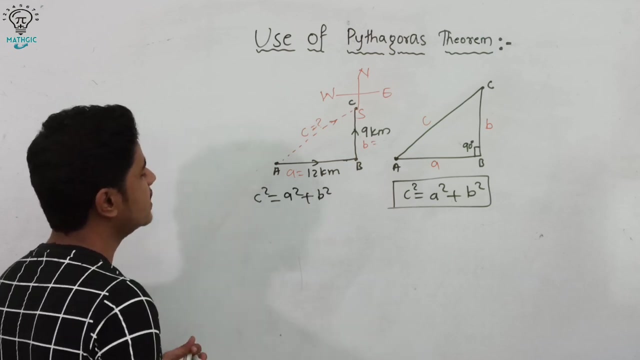 to reach a point C, We have to find distance from A to C. So this is C and that we have to find, and this one is A and this one is B. Now Pythagoras theorem says: C square is equal to a square plus b square. c square is equal to a square plus b square. where to find c square? 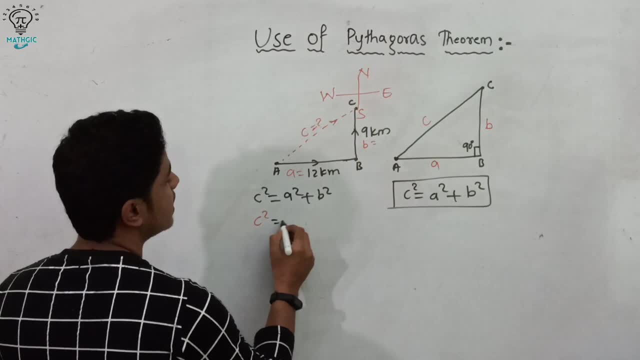 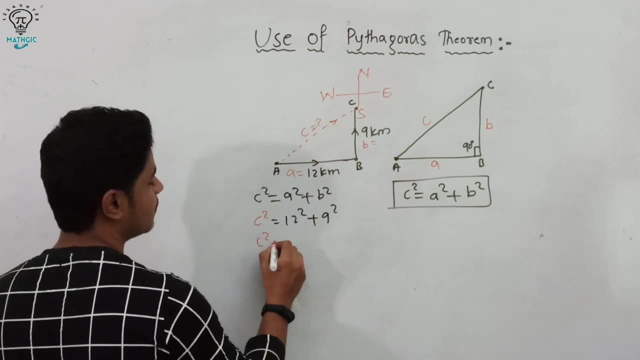 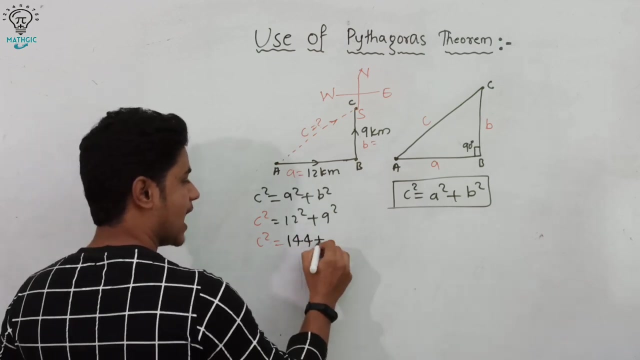 c square. now a square is: a is 12, 12 square plus b is 9. 9 square square means multiplication of same number to itself. c square is equal to 12, square is 12 times 12, 144 and 9 square is 9 times. 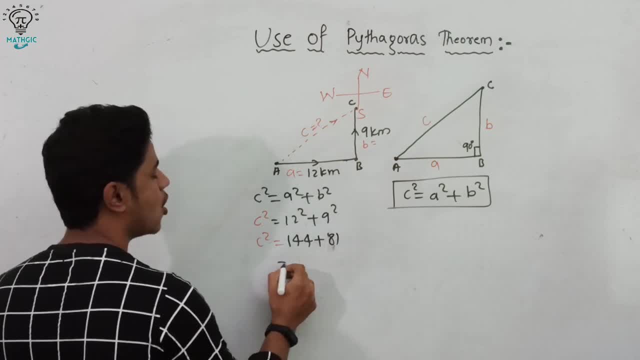 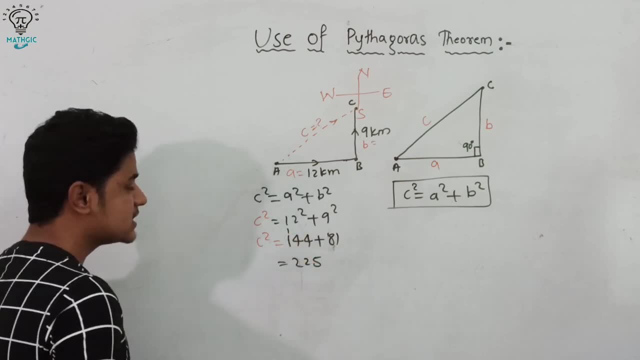 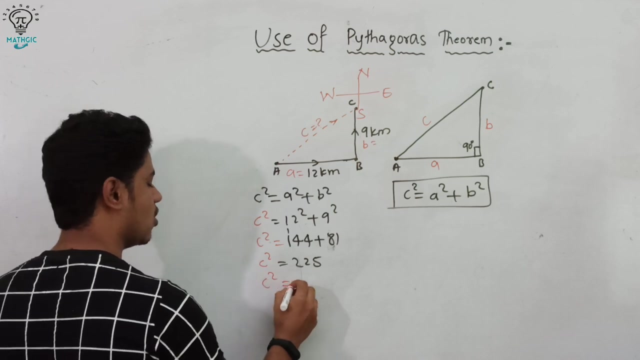 9 is 81, so 9 times 9 is 81. now add both 1 plus 4, 5, 8 plus 4, 12: 1 carry 1 plus 1, 2, so this is c square. c square is equal to 1, 225. where to find c? so c square is equal to 225. can be written as: